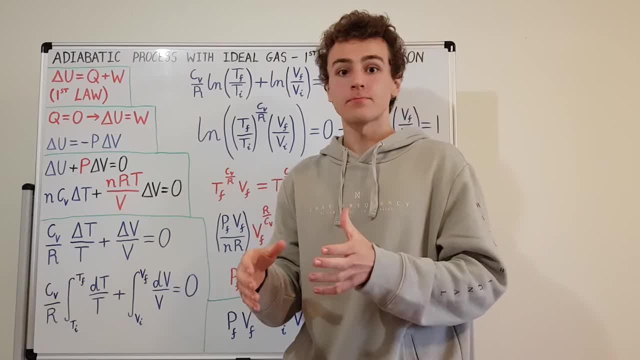 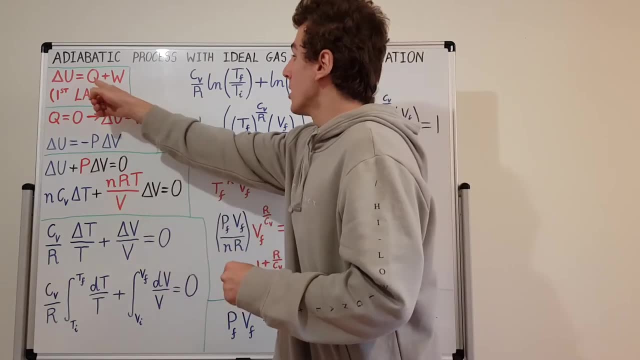 energy is due to either work or heat. Capital Q represents heat and capital W represents work. So we know that this is going to be zero, because it's an adiabatic process. There's no heat flowing in or out, So we can immediately say that this is an adiabatic process. So we can immediately say 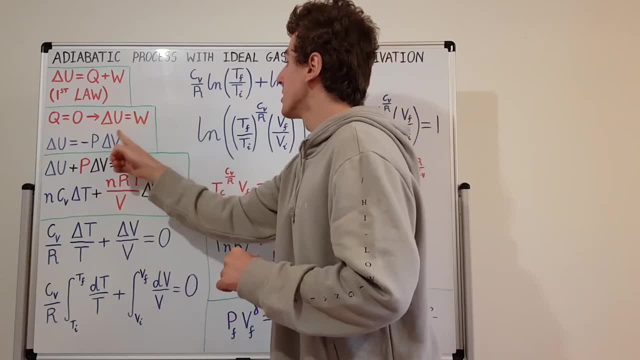 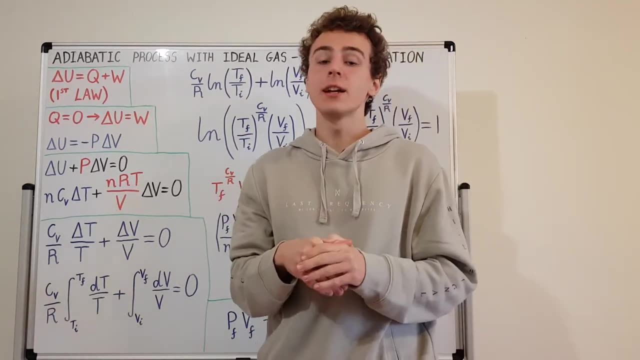 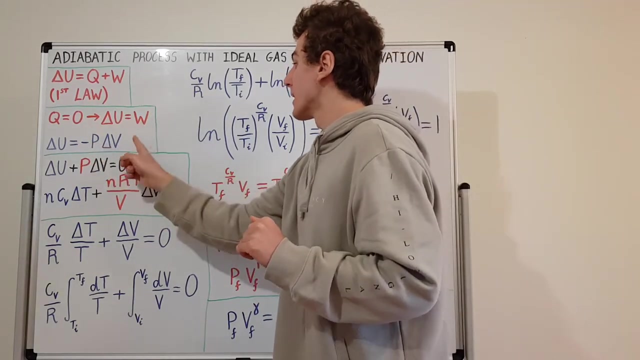 Q equal to zero. So now we have the change in internal energy is equal to the work. But what is the work In this scenario? we're only considering compression, expansion work. So that's given by minus P delta V. So this W, this work, is actually minus P delta V. Now why is there a minus sign? 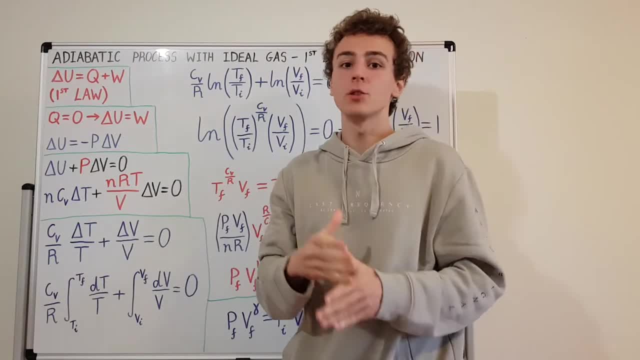 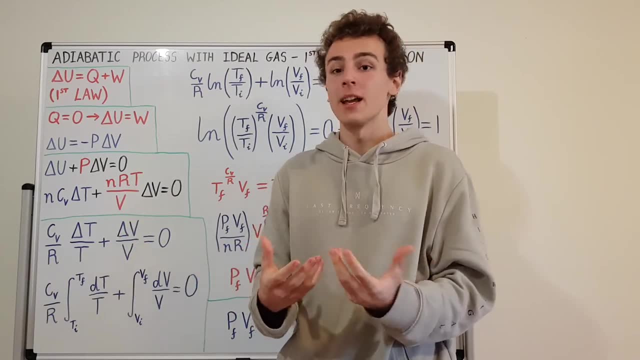 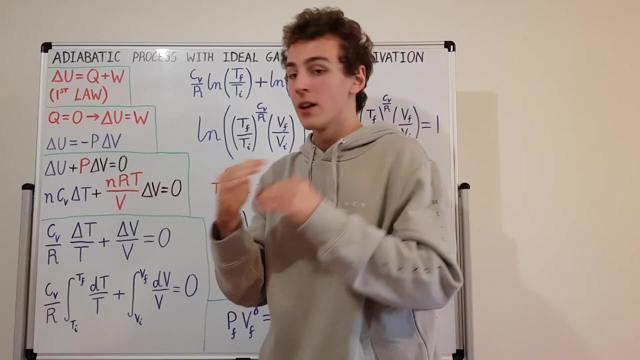 here. Well, the minus sign is by convention, because we're talking about the gas. If work is done on the gas, it increases the work. So we're only considering compression, expansion work. So if the work is done by the gas, it decreases the energy of the gas. So if this delta V is positive, 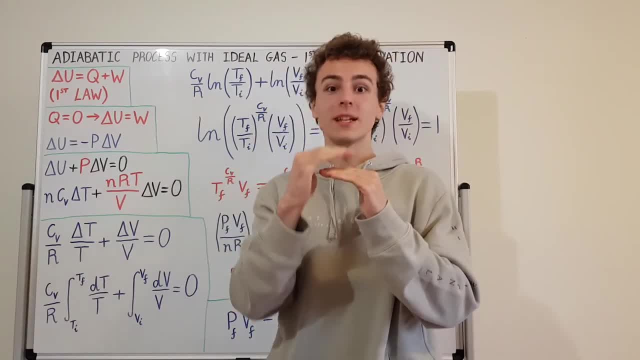 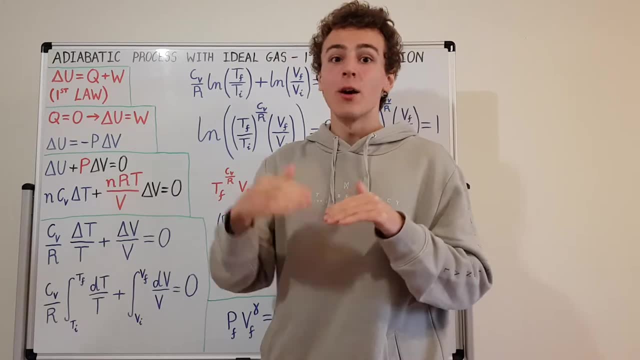 then we've got expansion right. Positive delta V means the volume is getting bigger, so we've got expansion. And if there's expansion, that means we have to put a minus sign because we're losing energy. We're losing energy with a positive delta V. What if it's a negative delta V? If this is? 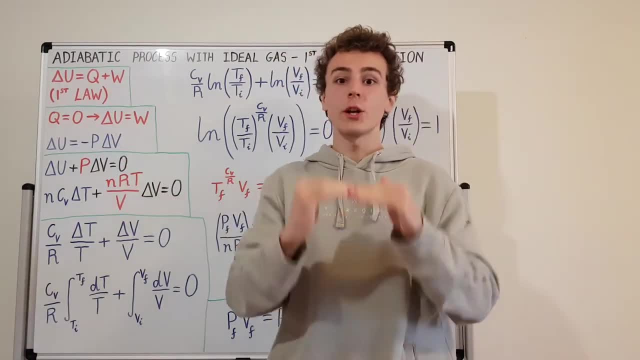 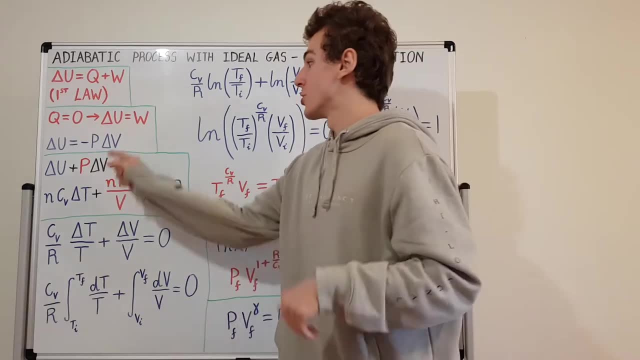 negative. then we're compressing, We've got compression, So we're only considering compression, expansion, And compression is associated with a gain in energy And a negative times. a negative gives a positive. So this convention is very useful for us. So keep in mind this negative. 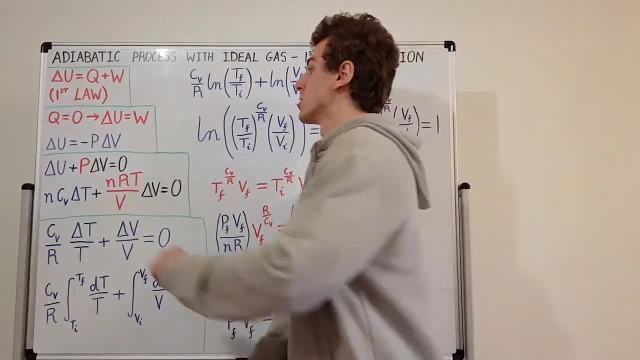 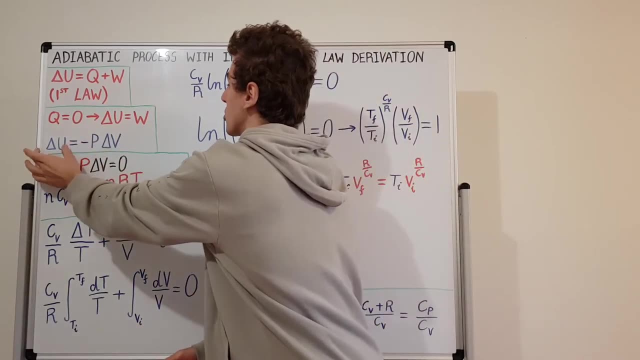 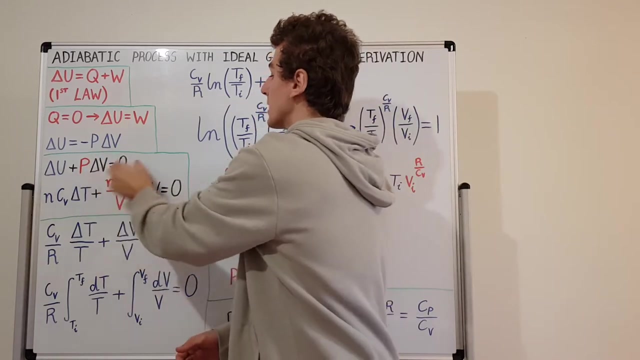 sign is here for convention purposes. So now what we have is the work where this expression for compression, expansion work is linked to the internal energy. Now what we can do is quickly add this to both sides of the equation And we can set this all equal to zero. Now it's going. 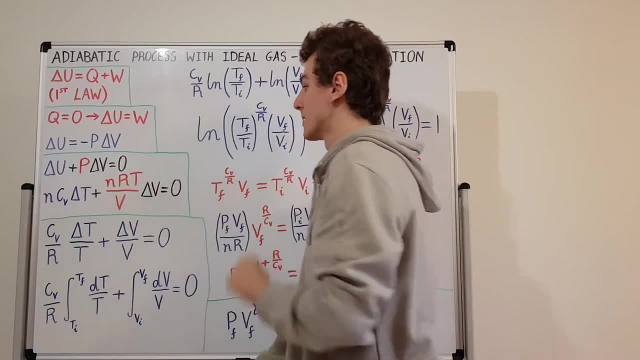 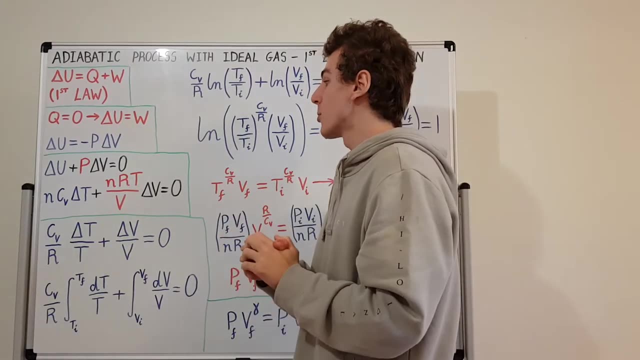 to become apparent why I'm doing this, why I'm setting everything equal to zero, because it's for a little trick that I'm going to implement later in the derivation. The next thing I want to do is I've color-coded some things that I'm going to substitute in here. So the internal. 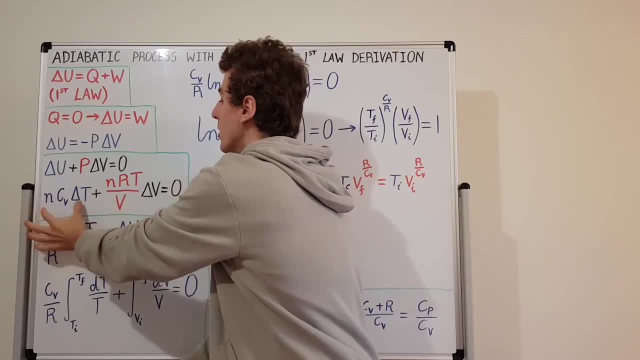 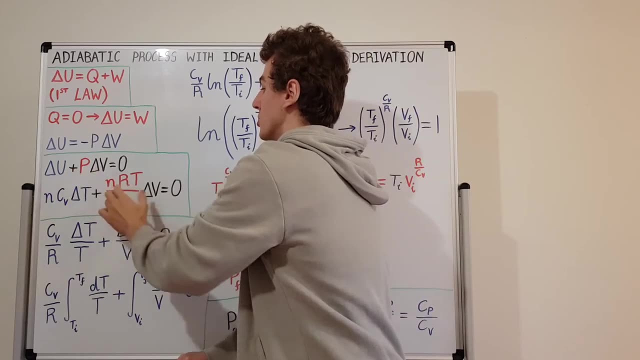 energy can be written with all of this blue stuff, So everything that's in blue. this corresponds to the internal energy. The pressure can be written with all of this red stuff and that corresponds to the pressure. So red over here and the blue over here are what I've substituted. 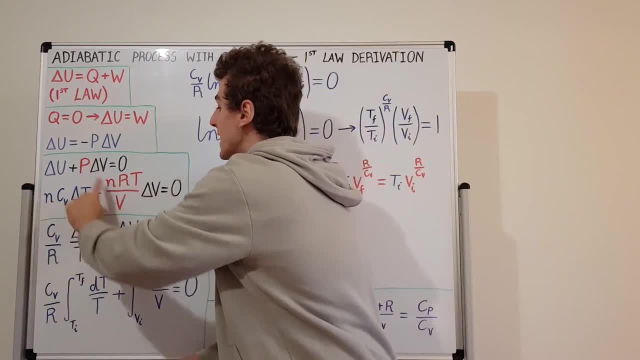 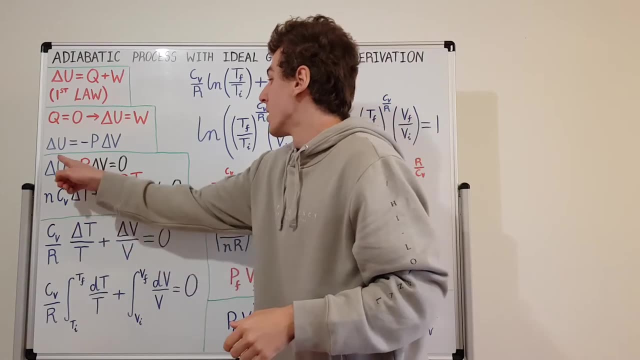 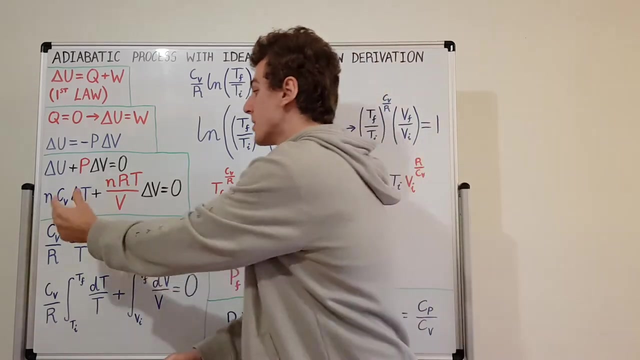 So this over here comes actually from the definition of heat capacity with constant volume. So nCV delta T, that tells us the change in internal energy. This works for an ideal gas. it doesn't necessarily work in general. So this is actually saying that the change in temperature 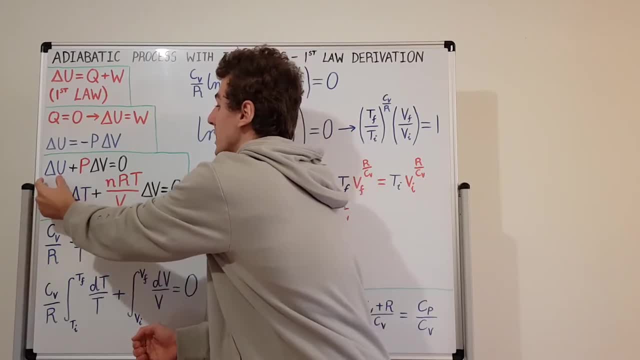 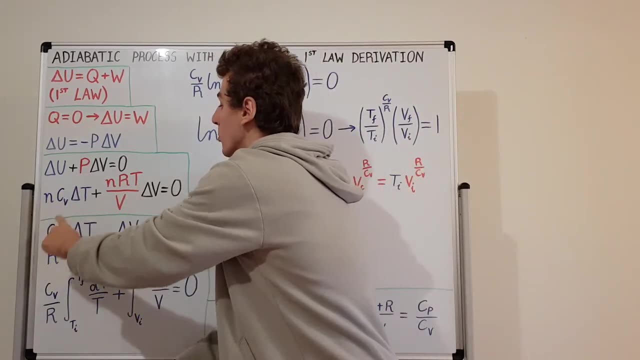 has a direct correspondence with the change in internal energy. This is for an ideal gas, So Cv and n are the constant with constant volume. So this is actually saying that the change in temperature, which tells us how a delta T can give us a delta U, So a change in temperature. 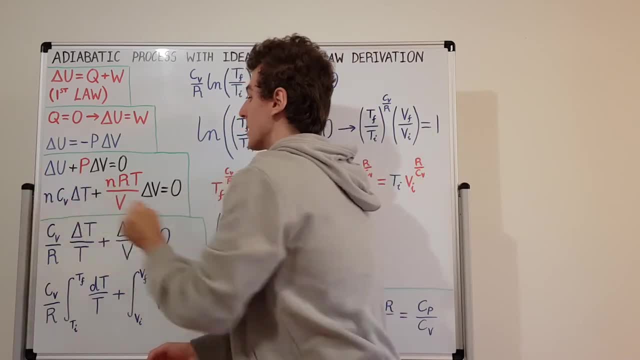 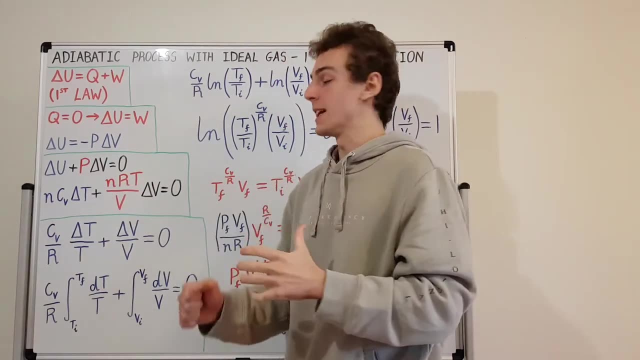 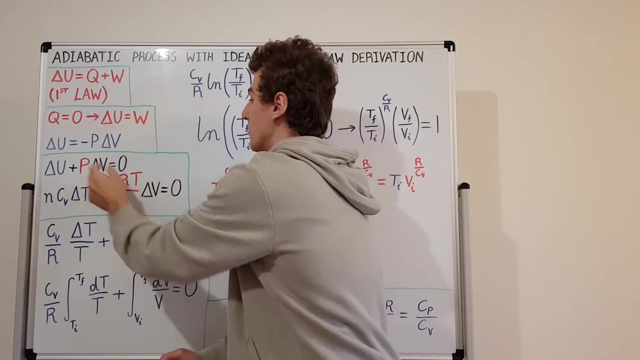 causes a change in internal energy. So that's this first term that I've substituted in. The next bit over here is invoking the ideal gas law: PV equals nRT, Where this is a slight rearrangement: P equals nRT divided by V Right. That's what this is actually saying. 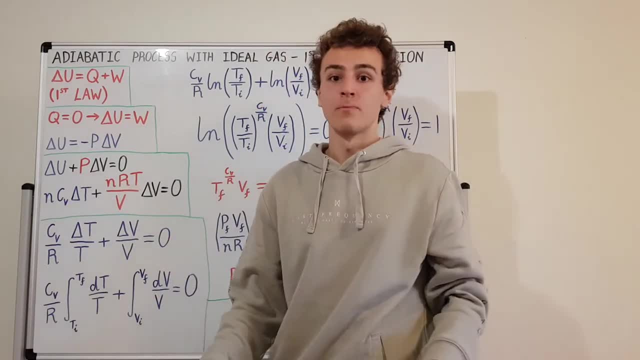 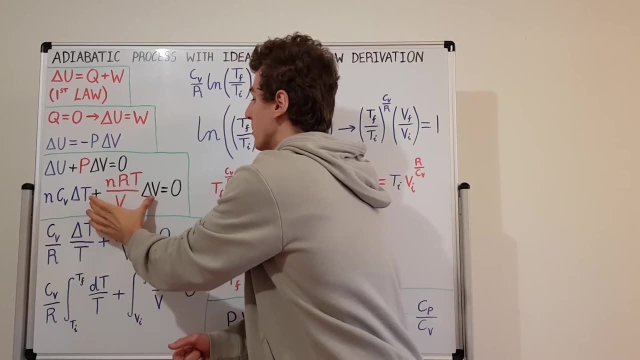 P equals nRT divided by V. That comes from the ideal gas law, And that's the first time we're invoking the ideal gas law in this derivation. So now we have this condition. All of this plus all of this sums up to zero. 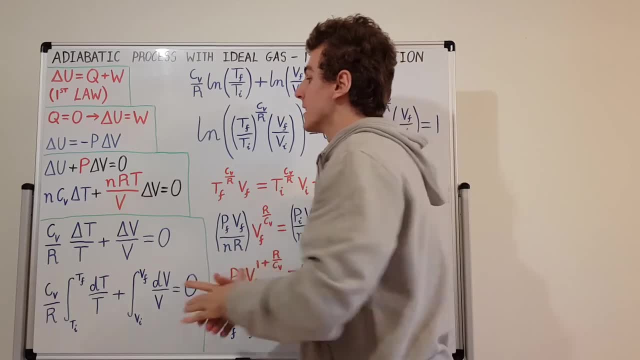 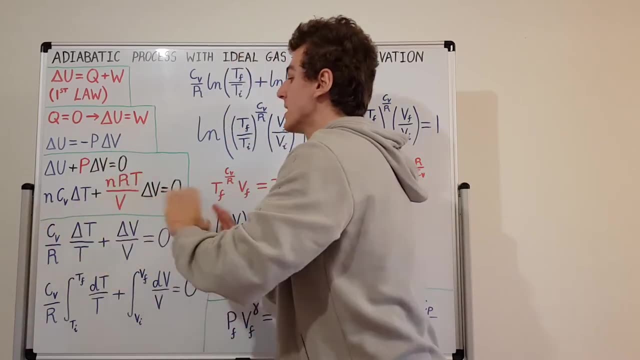 That's what this condition is saying. Now we can do is we can see that there is an n. This n is the number of moles. We can actually cancel this out because this property is independent of the number of moles you have of the gas. 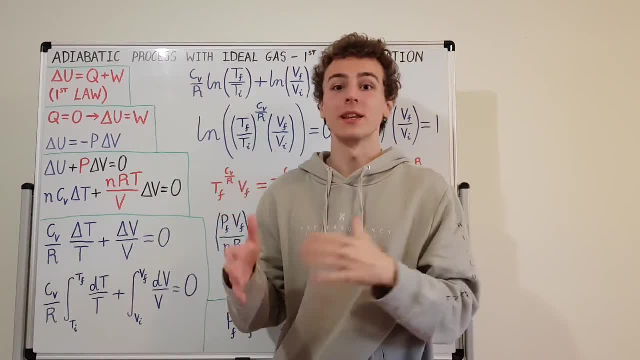 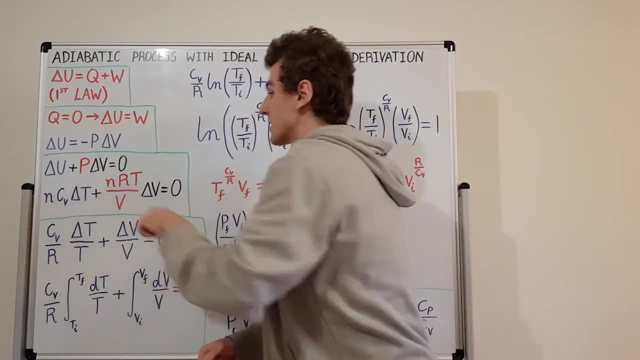 So the amount doesn't actually determine the condition, which would make sense. The same condition holds regardless of how much gas you have. So this we can cancel out. Then what we can do is we can actually divide by RT, so we can divide by R and 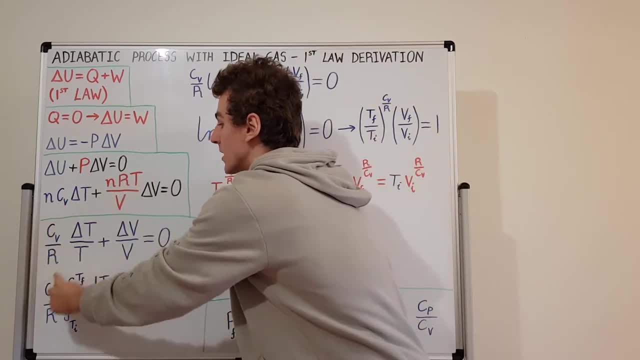 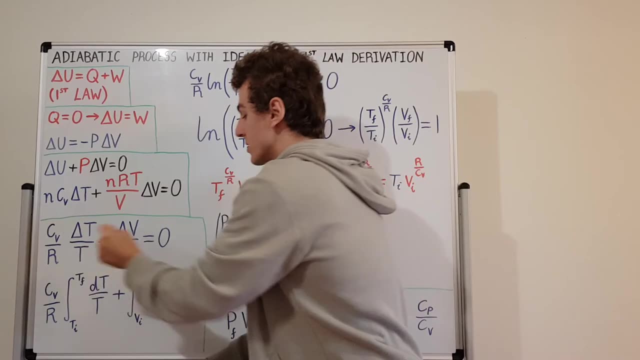 divide by T, If we divide by R, we get this constant over here on the left term. And if we divide by T, we have this Delta T over T And you can see there's a Delta T over T and there's a Delta V over V. This over here, this condition is: 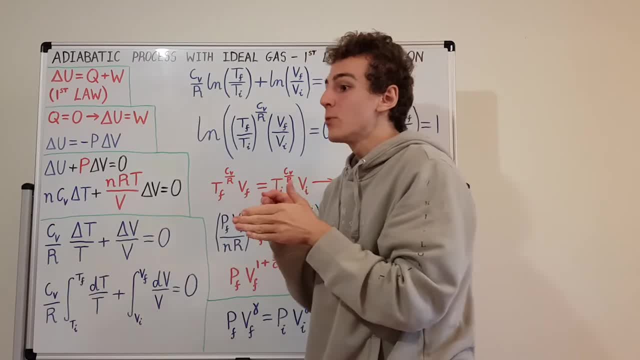 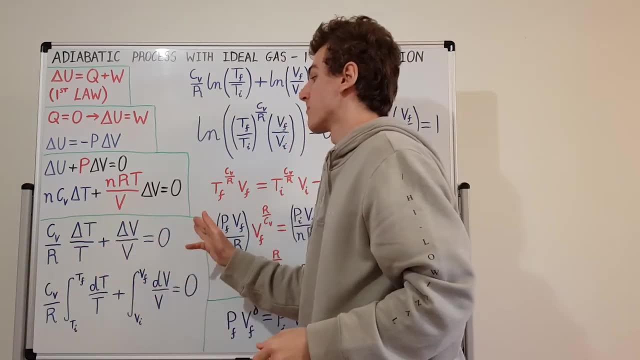 for a tiny little change in, a tiny little nudge in the temperature at a tiny little Videos in the description, nudge in the volume during an adiabatic process. That's what this is describing. But what do we know that can help us add up a bunch of tiny little nudges? 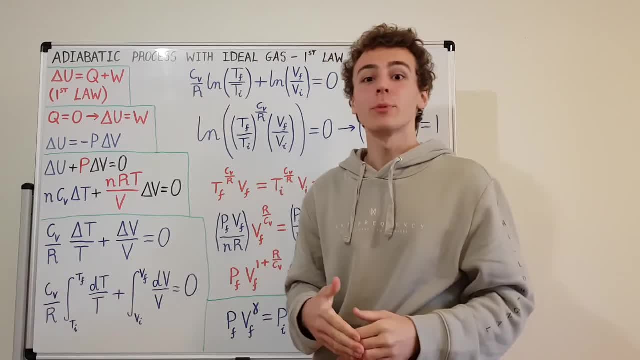 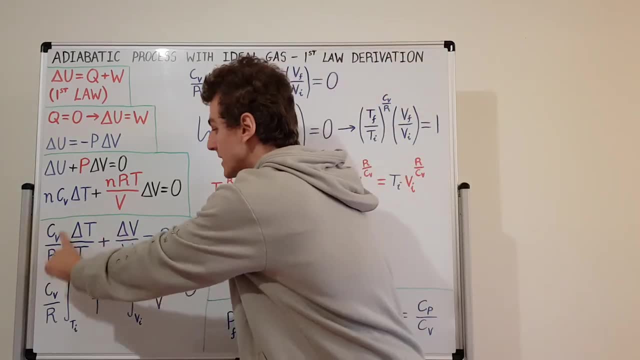 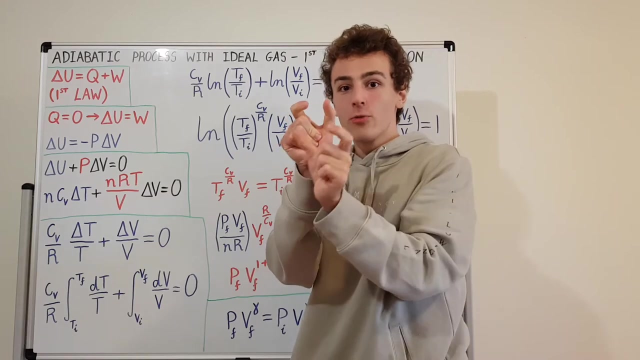 Well, integration, Integration in calculus, can help us add up tiny little changes together. So it's the cumulative effect of many, many tiny little changes. And when we see this kind of relationship over here, immediately we should be thinking natural logarithm, Because if you have a tiny change over the quantity and you add that up, 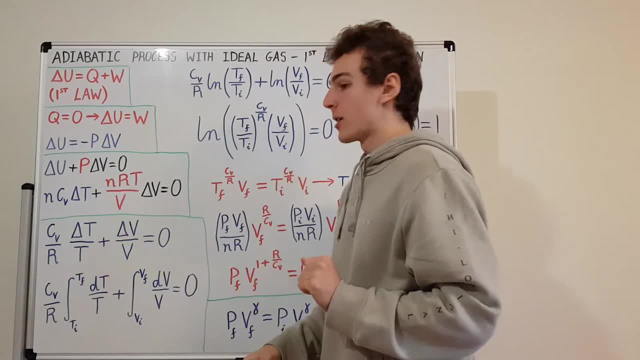 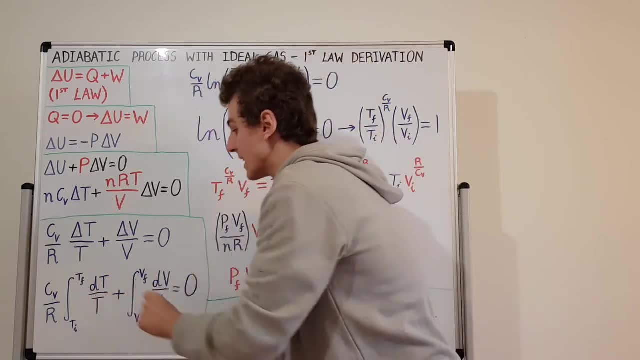 you're going to get the natural logarithm. Let's rigorously see where that comes from. So what I've done over here is I've changed this little delta. it's no longer a little change, it's now a dt, so it's a differential. And here we have a dv And we're integrating these guys. 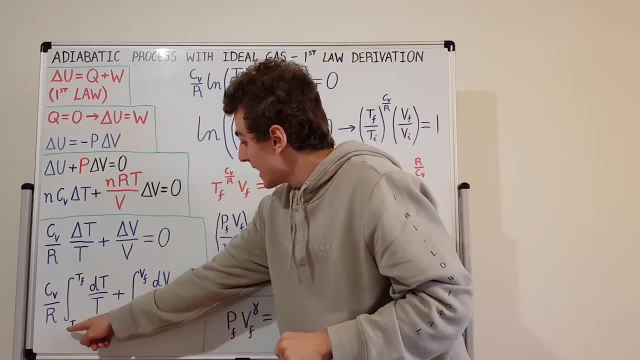 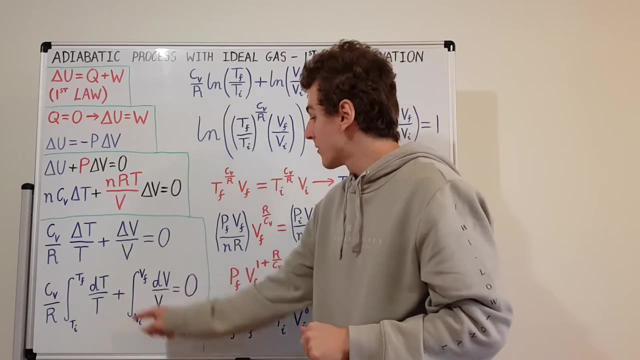 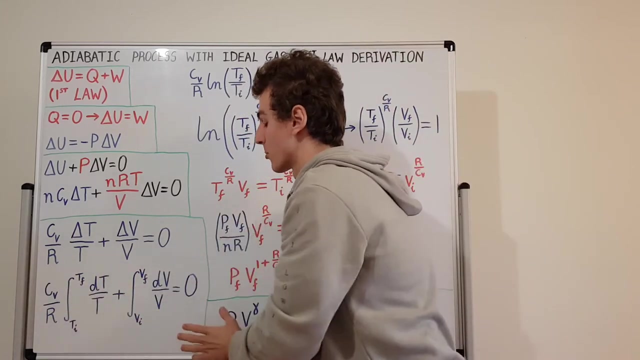 from the initial to the final state. So the initial state is ti, the initial temperature, And the final state is tf, which is the final temperature, And we also have the equivalent expression for volume, which is from vi to vf. So now we can actually evaluate these integrals. And if you're familiar with 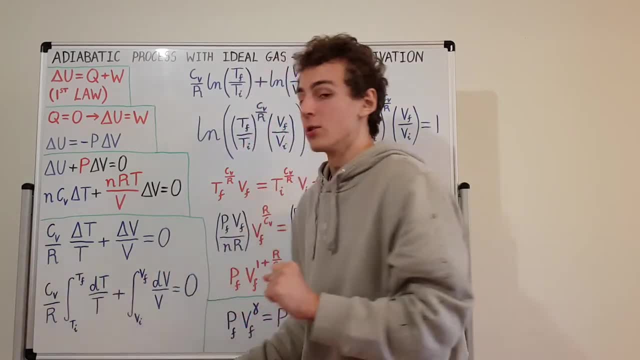 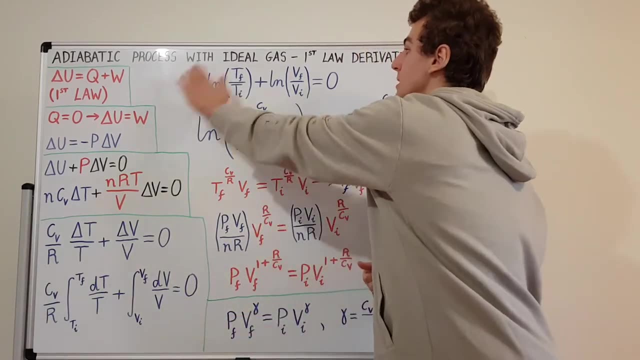 single variable calculus. you'll know that this is the natural logarithm. So the integral of 1 over x is ln x. So let's have a look at this expression over here. This is what happens when you evaluate these integrals. you get these two natural logarithms. 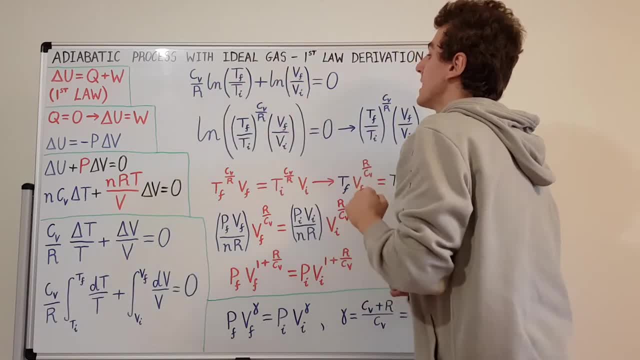 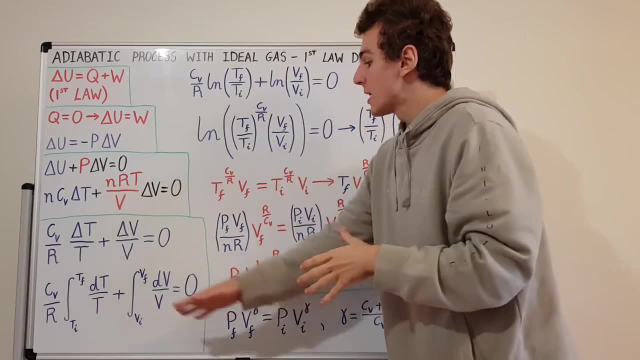 Now, why is there a ratio of tf over ti and a ratio of t over invited? And of what? of vf and vi? Well, these ratios actually come from evaluating the integral. So if you kept it as an indefinite integral, you would just get natural. 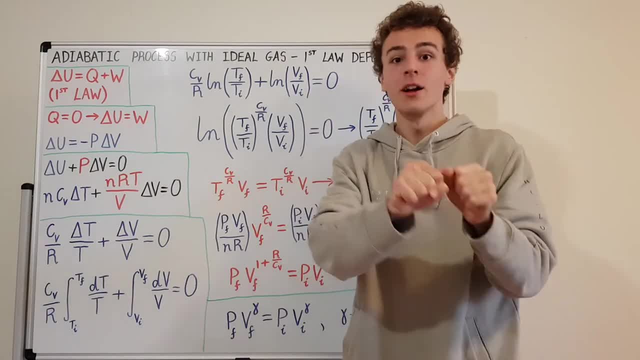 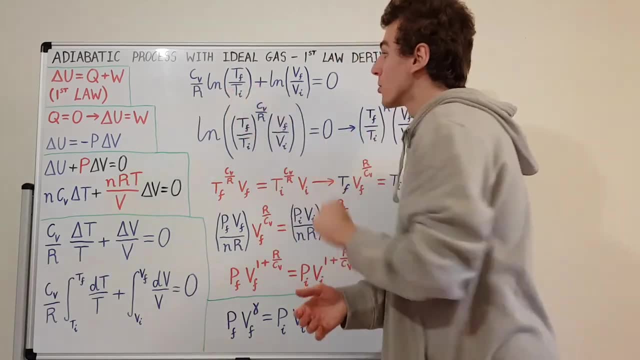 log evaluated from the final minus the initial. Right, you'd have the difference between those guys, the final minus the initial, And we can actually use log laws to just combine that. You have final minus initial. well, if there's logs acting on those guys, then that turns into log. 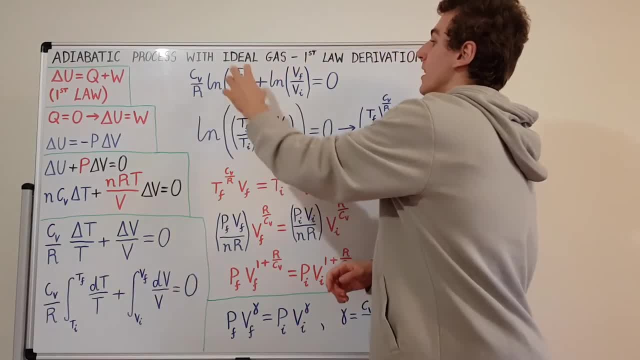 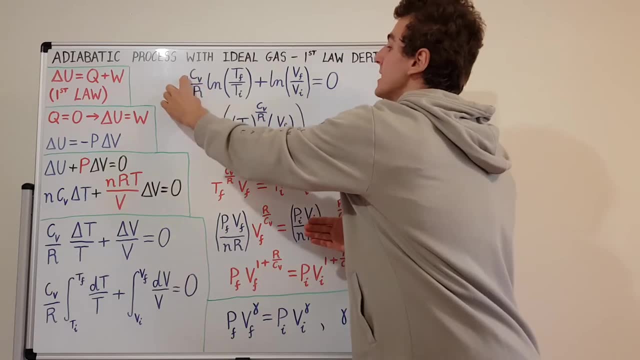 because if you kept it as direito and I kept it as integral, you would just get natural log evaluated from the final, have a log of a ratio and that's what we see. these two guys, The ratios, are inside the natural log. Now we can use some more logarithm laws and we can take this: 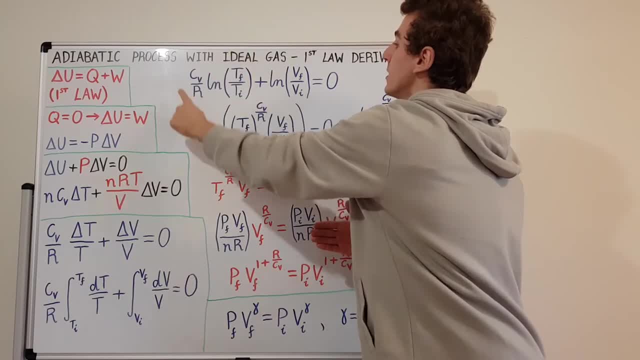 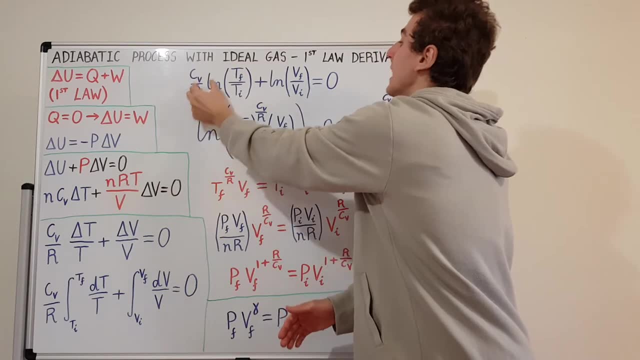 exponent and we can bring it upstairs over here. So this exponent or this coefficient can actually turn into an exponent. right, If you have a coefficient multiplying this log, you can move it inside the log and then you can raise whatever is inside the log to the power of that coefficient. So this CV over R is: 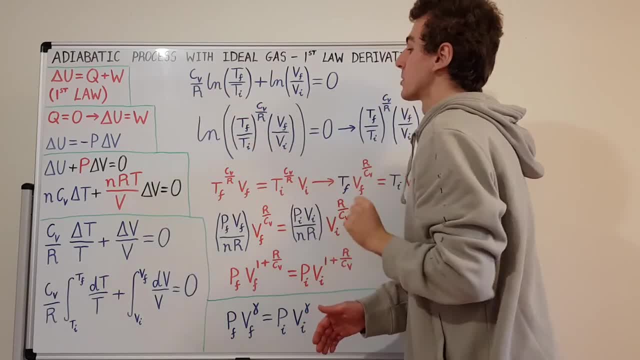 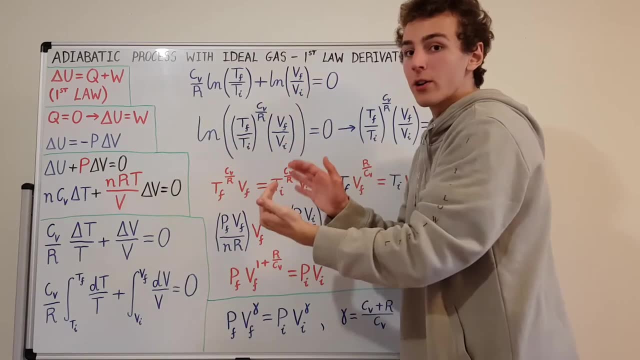 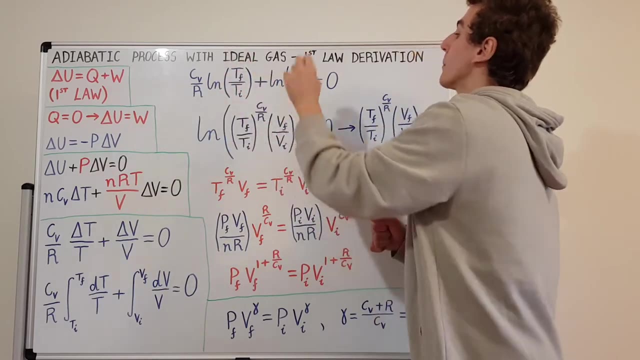 now the exponent of the ratio of the final and initial temperature. And what we can also do is when you have the sum of two of these guys, you can combine them into one log by multiplying whatever is inside. So we have this guy multiplied by this guy, because the natural log of this guy plus the natural 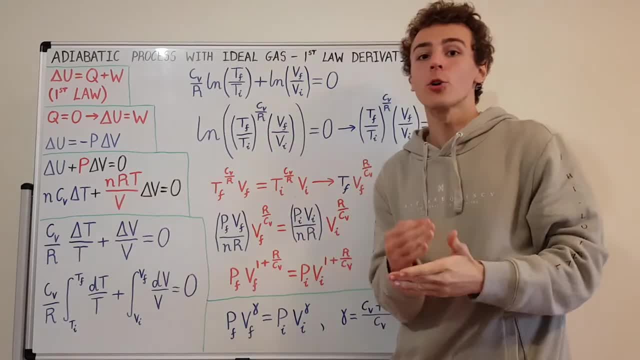 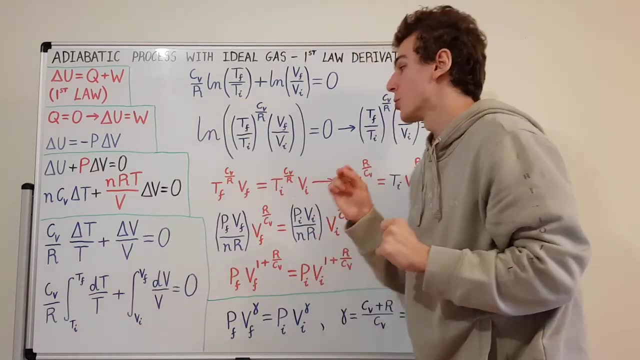 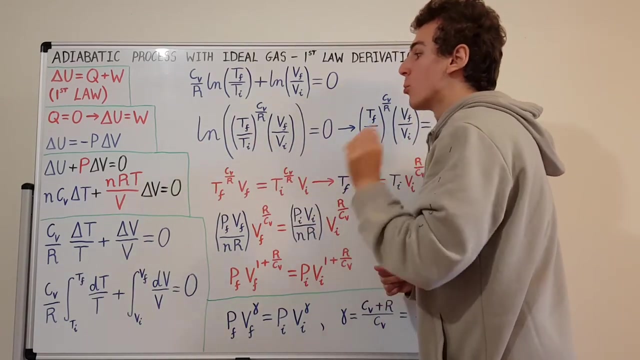 log of this guy is equivalent to this. So that's logarithm laws, And keep in mind we're dealing with a natural logarithm. That's log base E, where E is Euler's number. That's what this Ln means. This is Ln natural logarithm And now we can use. 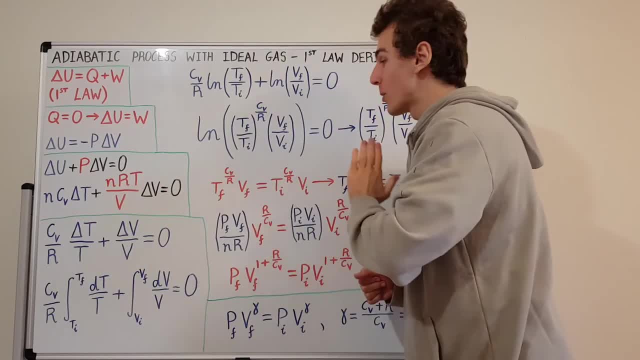 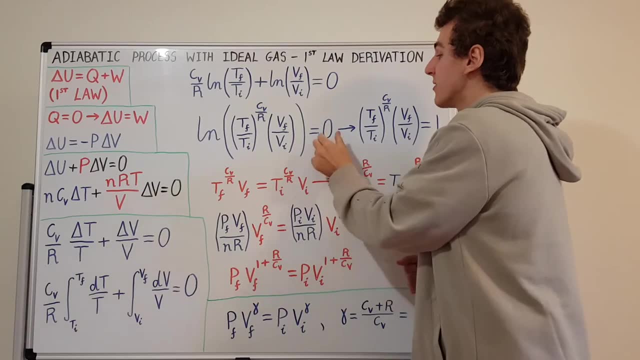 this little trick, that we've set this equal to zero, right? Remember, back in the beginning I said I'm going to set this equal to zero because I want to implement a little trick. And here's the trick I'm going to implement. If this is, 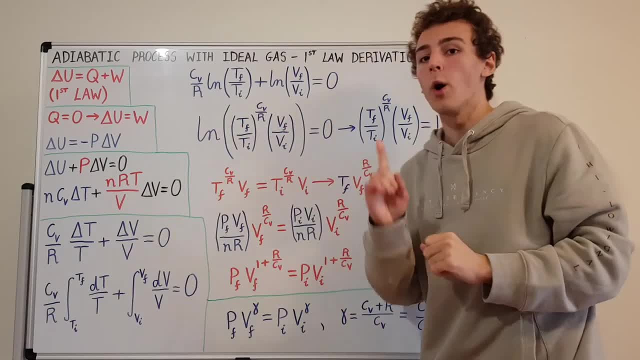 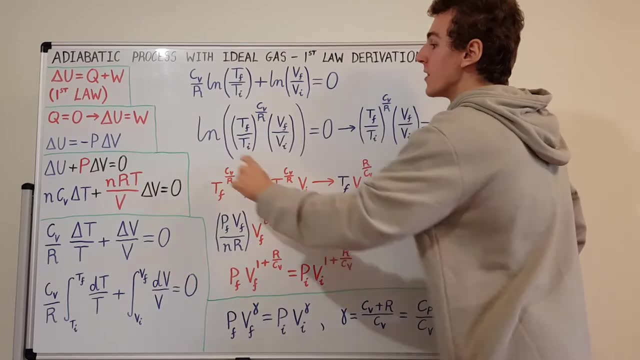 equal to zero, then we can infer that the inside is equal to one. right, We can infer this condition. How can we infer that? Well, what is this actually saying? If we rewrite this, this is the base over here, the implicit. 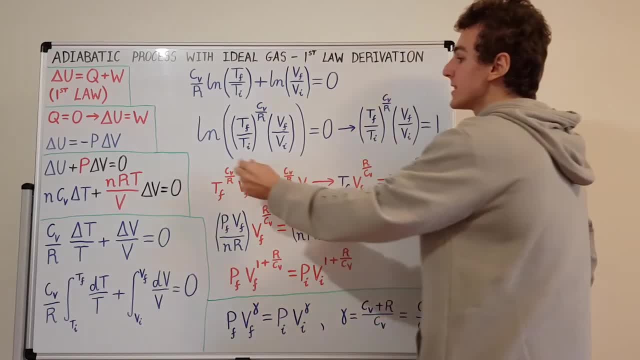 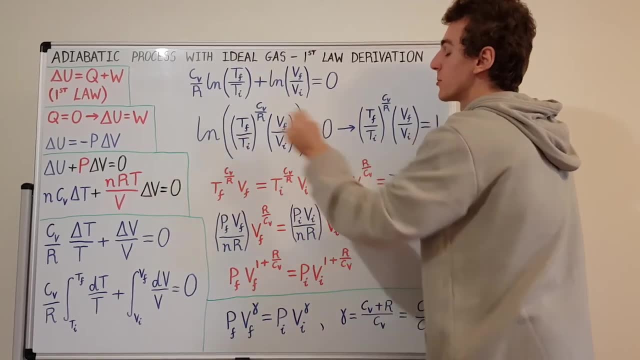 base is E, which is Euler's number. So this is saying E to the power of zero is equal to everything inside the logarithm. E to the power of zero is equal to that. So this is equal to E to the power of zero. E to the power of zero is equal to: 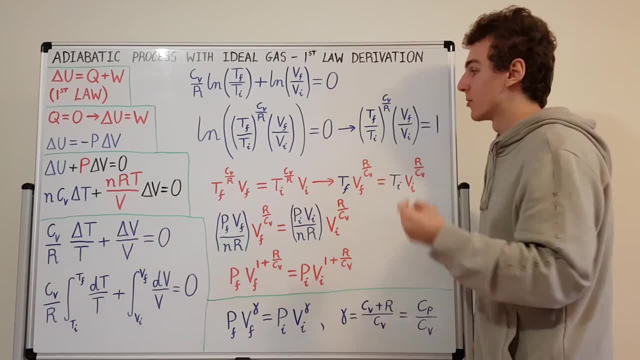 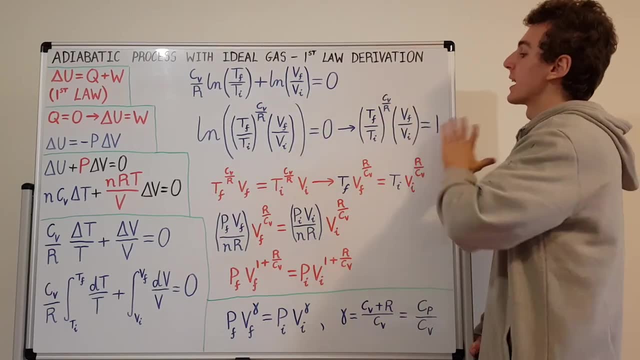 one, because if you raise any of these real numbers to the power of zero, you're just going to get one. So that's what this is. So E to the power of zero is equal to one, and that's why we can get this expression, And this is a very useful expression. 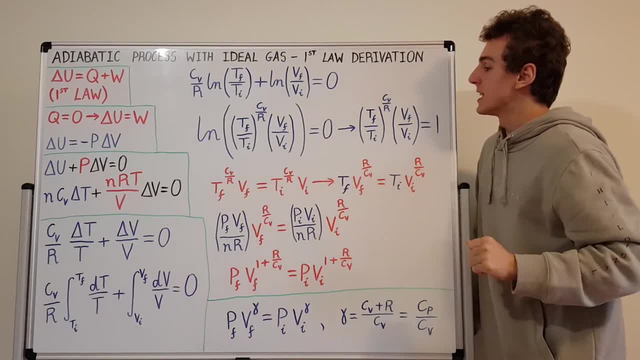 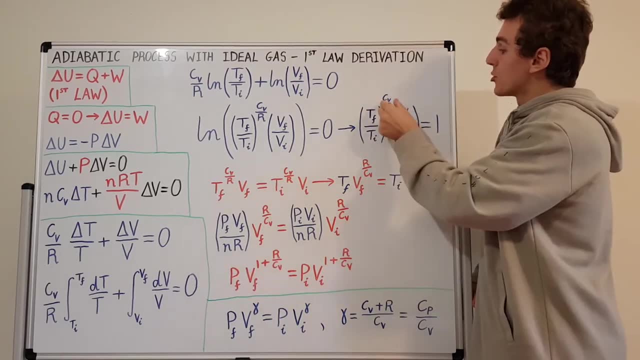 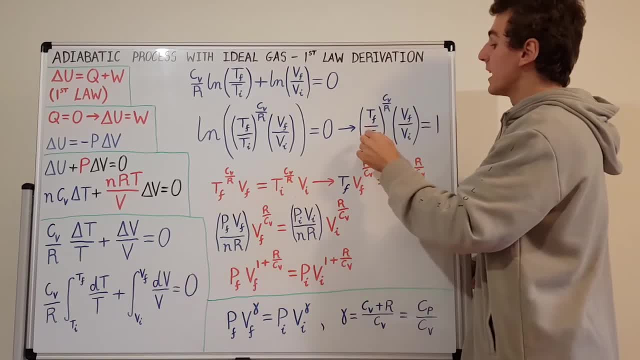 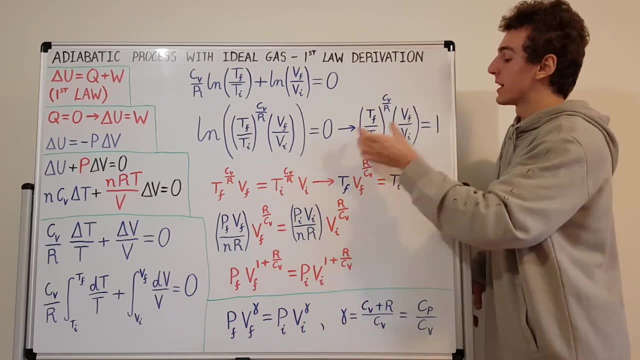 these guys. what can we do? Well, we can actually move this guy to the other side of the equation, so we can multiply both sides, right, Because this is just a 1, and if we multiply that by 1, we're just going to get whatever we're multiplying. 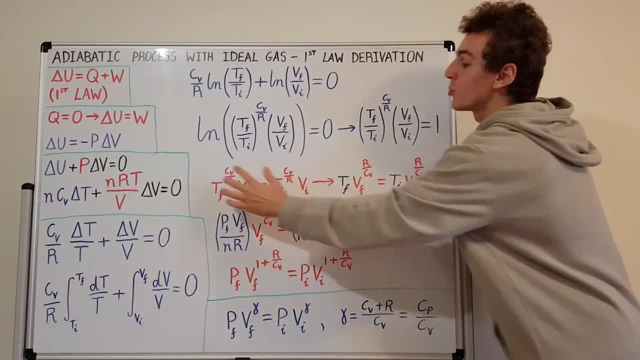 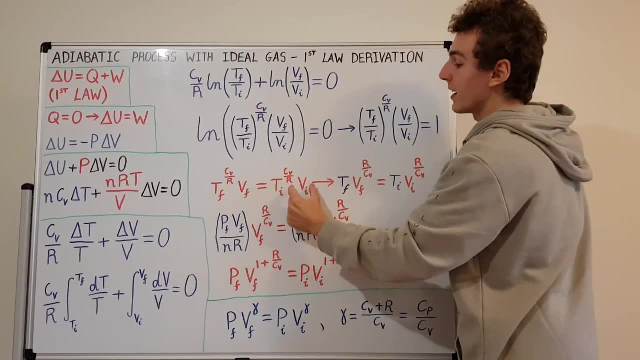 by then we can also move this Vi, and that's where this condition comes from. So you can see that this Ti was actually downstairs over here and this Vi was downstairs over here. So these guys you can actually divide back and you can get. 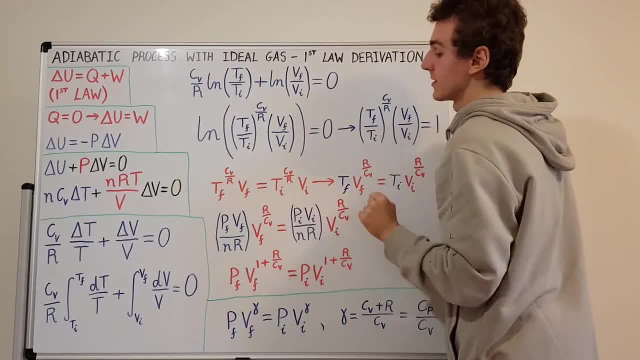 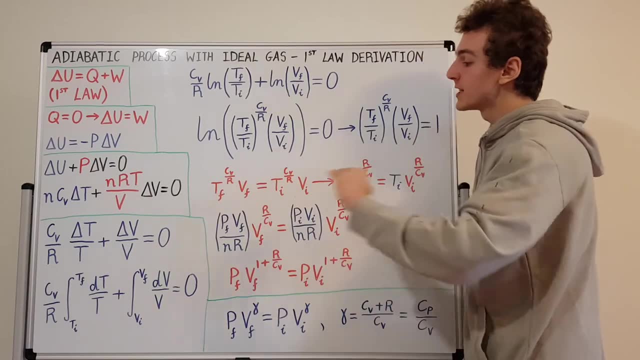 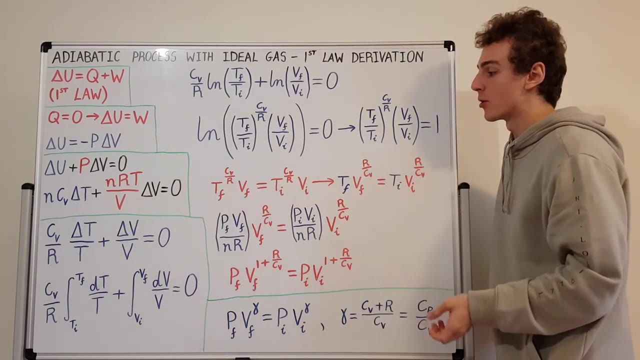 back into this condition. So this turns into this. What this is saying is that the temperature raised to this exponent times the volume. that is a constant value. But we don't want something in terms of temperature and volume. What we want is something in terms of pressure and volume, because we want to draw this on a PV diagram. 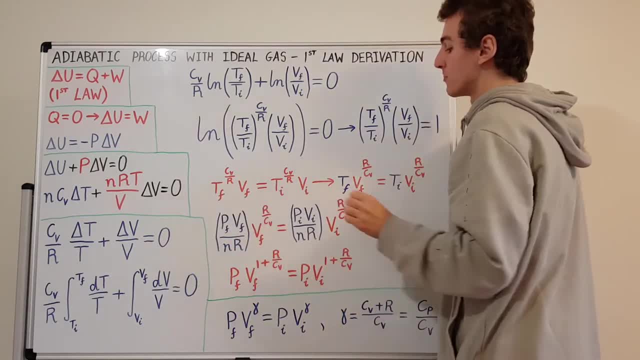 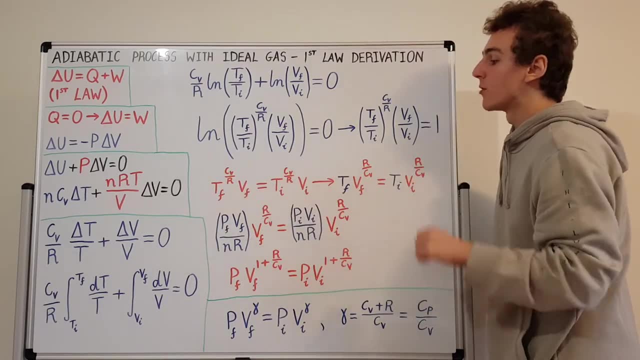 We don't want to draw this on a TV diagram, So what we can do is we can use another little exponent trick and we can raise both sides to the power of R over CV or the power of the reciprocal of this guy, and what that's going to do is when you 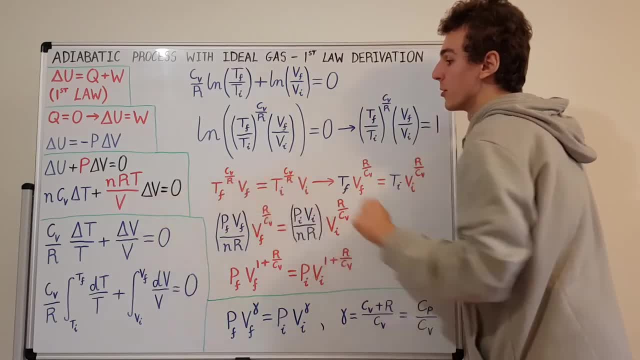 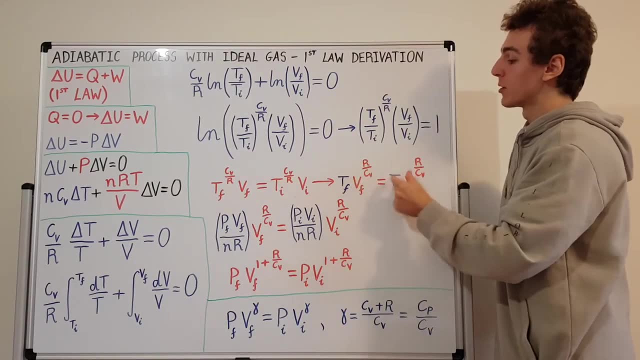 Apply the reciprocal of this guy to the, the temperature term It's going to cancel out, and the power you're going to get is 1. So you're just going to get 1 on these temperature terms which I've labeled here in blue. And if you multiply this 1, right imagine, 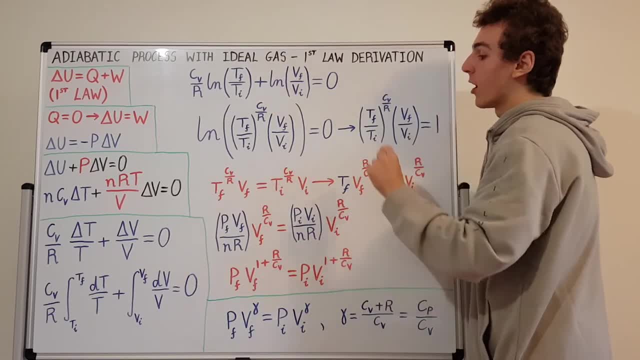 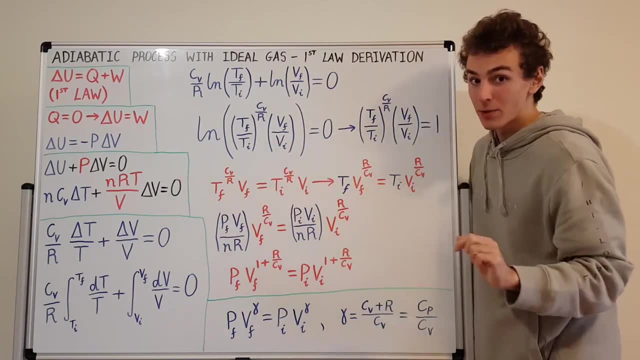 There's a, there's an implicit 1 above this V by R over CV. Well then, you're just going to get this guy. So what is the end result? Well, you just flip the fraction, take the reciprocal and you move it to the other guy. 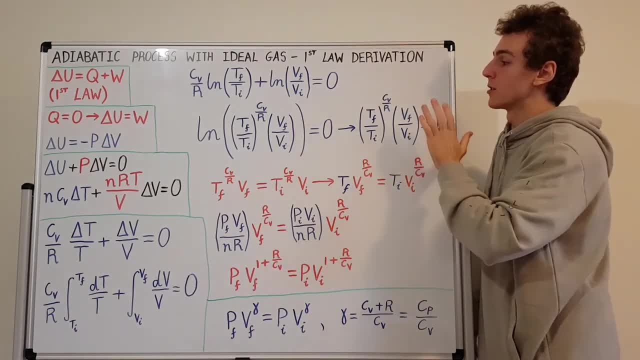 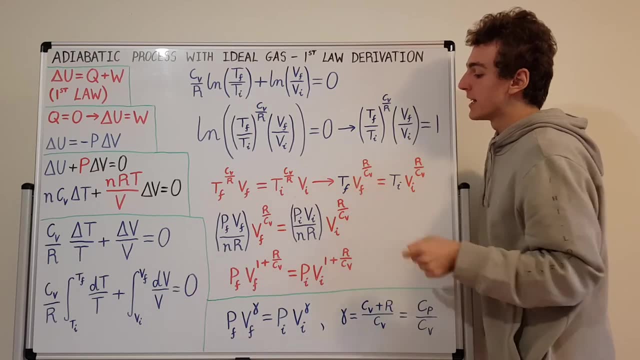 This is valid from exponents laws. So we've used logarithm laws and now we've used exponent laws. So now we have this condition. So now we have this condition. Now, why have I transferred the exponent from the temperature to the volume term on both sides? 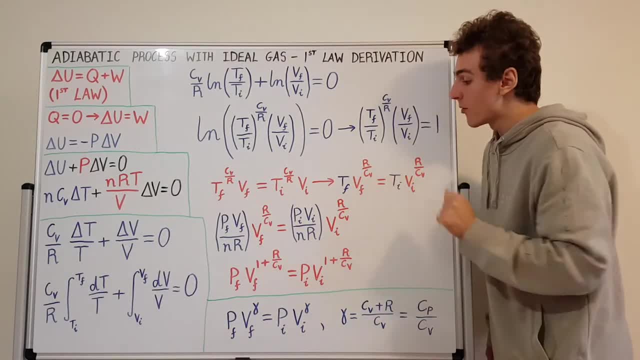 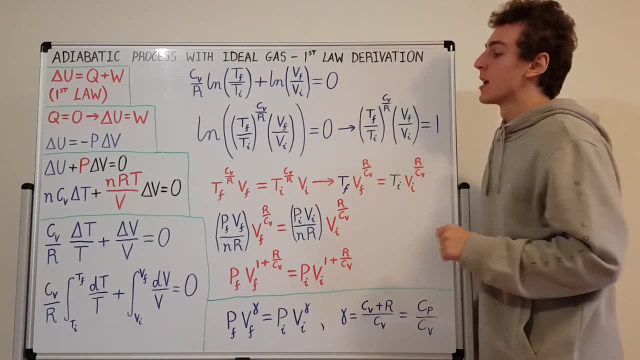 Well, it's because I want to get rid of this temperature. I want to keep the volume, but I want to get rid of temperature. How can I get rid of temperature when I can invoke the ideal gas law again? So I invoked the ideal gas law back over here in this red expression, right? 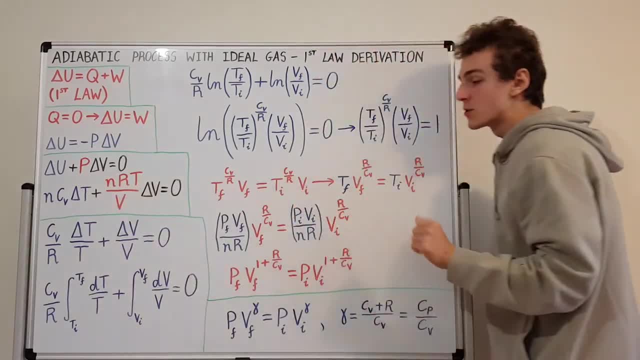 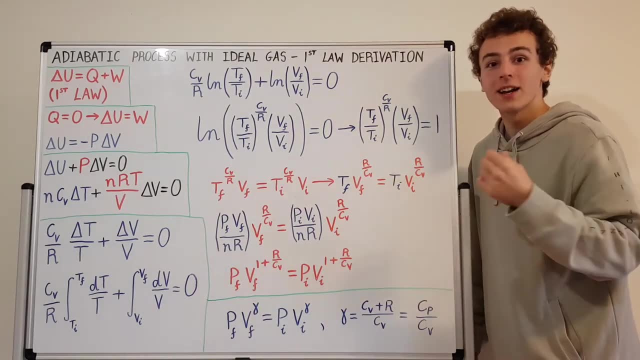 I said P is equal to n RT. on V, that comes from: PV equals n RT. Well, we can do another manipulation and we can see that T Is equal to PV divided by n R. so this fraction, P times V over n R is the same as T. 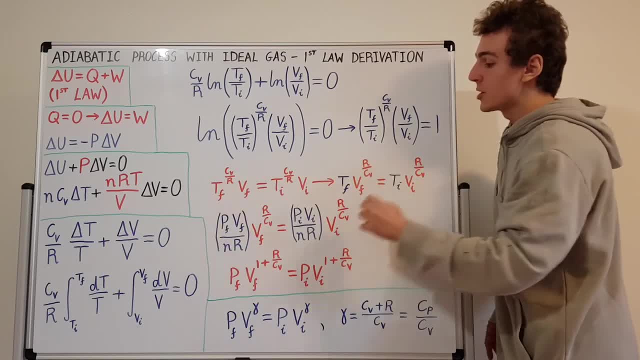 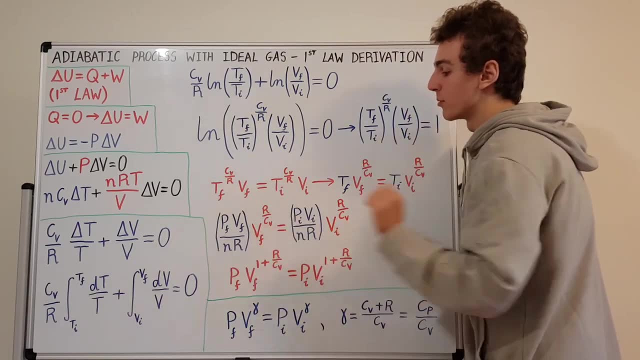 So we can substitute that in for the final state and the initial state on both sides. and have a look: there's n R on both sides. so that means we can cancel n R on both sides, and You can also see that there's one P on both sides. So that just remains. 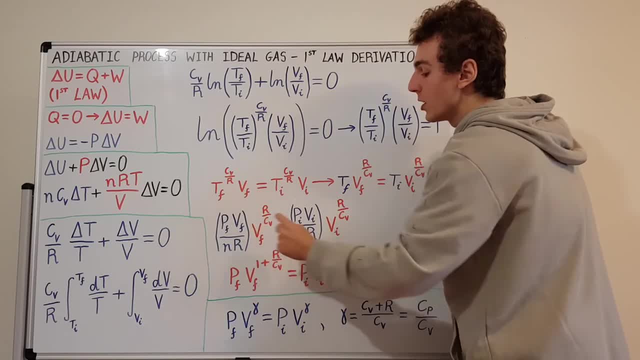 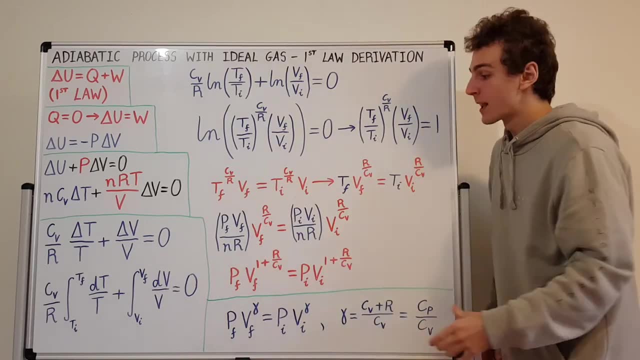 We just have one P and we also have one V over here and we have a power of R on CV over here. So what we can do is we can again use an exponent law, Because this is the same base on both sides, and we can add the exponents when we multiply these guys together. 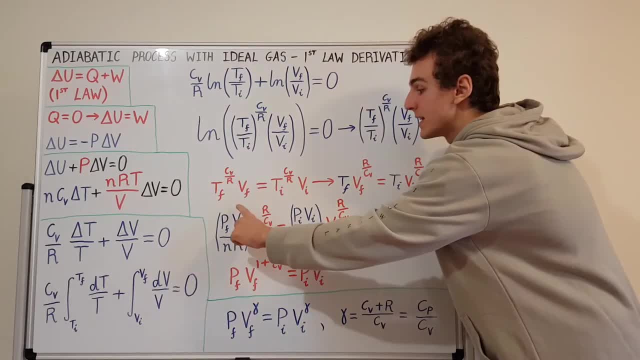 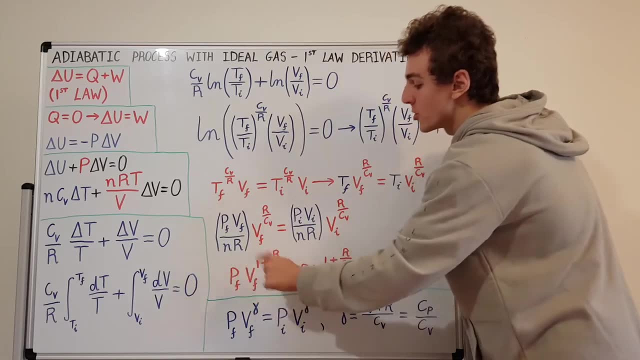 Right, if we want to multiply them together, We add the exponents. the exponent of this is 1, so we have 1 plus R on CV and that is the exponent over here. So now we have something in terms of pressure and volume and some magical exponent. Let's rearrange this magical exponent. 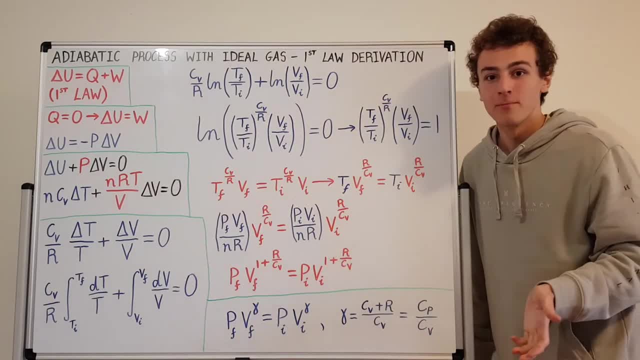 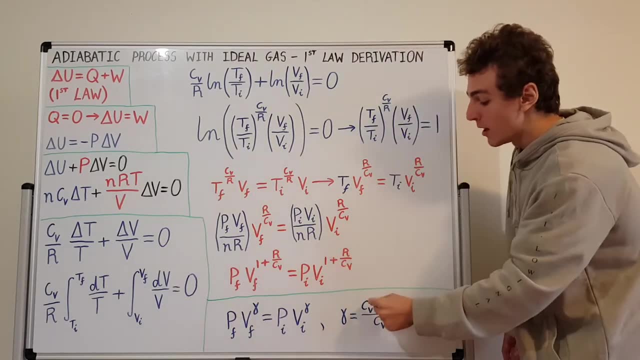 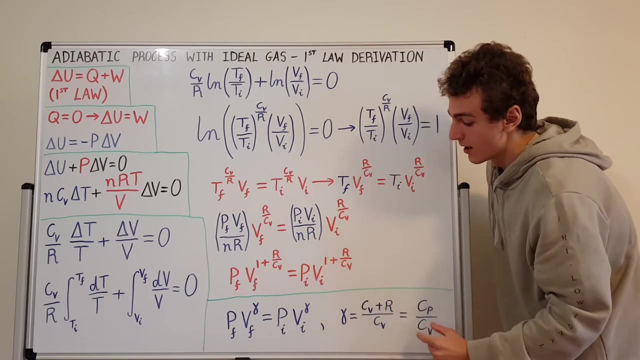 Let's turn this 1 into CV divided by CV, so we have a common denominator. If we want a common denominator, What we can do is we can have CV plus R on CV. So if you turn this 1 into CV on CV, you get this right- this expression- over here. 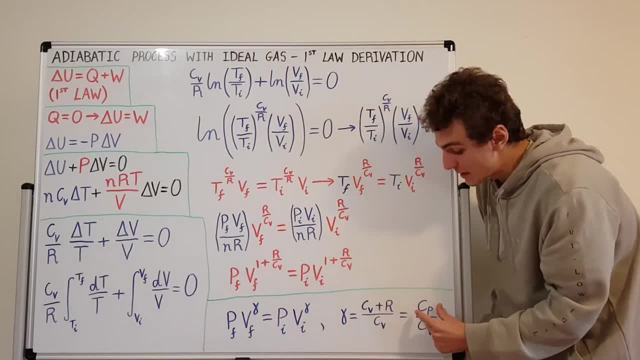 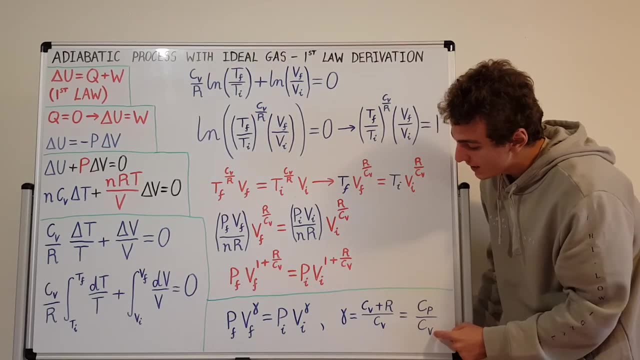 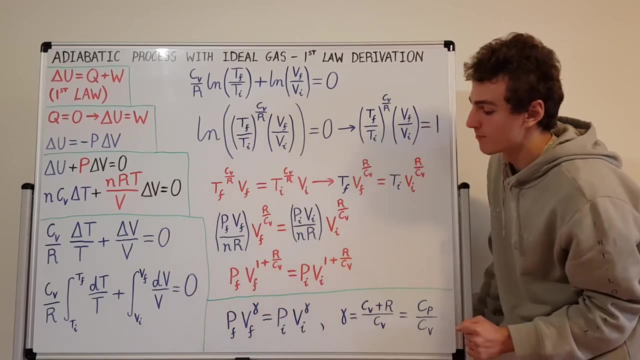 But what is CV plus R? Well, that's CP, right for constant pressure, That's the heat capacity for constant pressure, and the ratio of CP on CV That's defined as gamma, and this exponent goes on the volume on the volume term over here. isn't that fantastic. now we have a 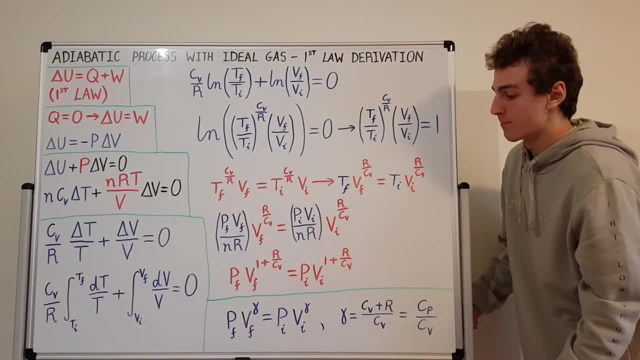 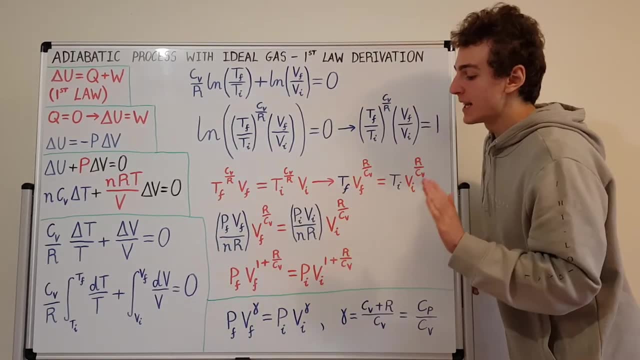 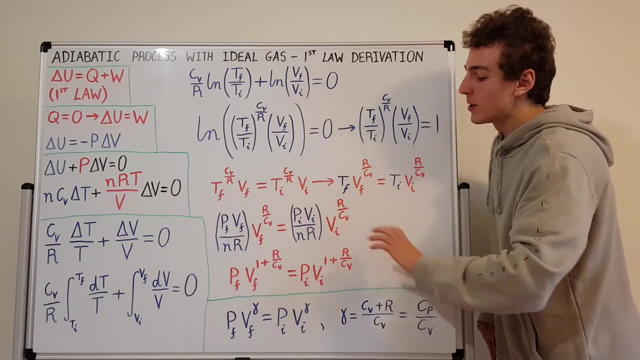 Relationship between the pressure and the volume for an adiabatic process. We could have stopped over here, Right, This is also a relationship, but it is not a relationship that has pressure and volume. You can rewrite this in terms of pressure and temperature. You can keep substituting the ideal gas law and manipulate and get a bunch of different combinations. 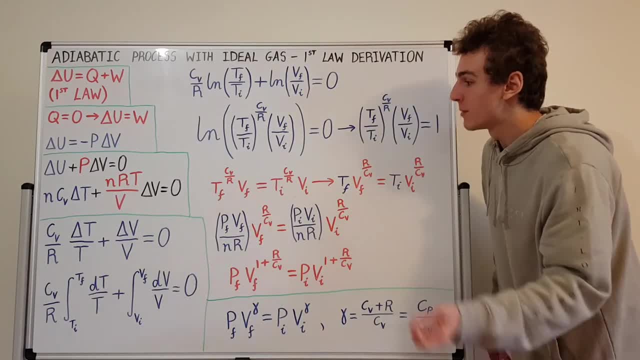 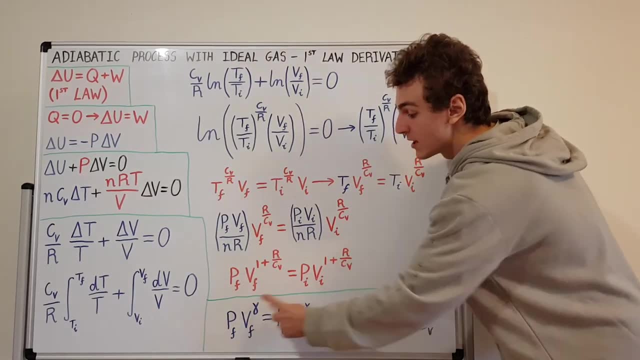 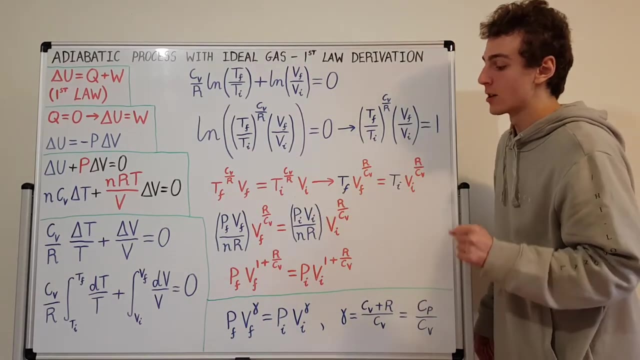 You can have pressure, temperature, pressure volume, temperature volume, do a bunch of these combinations and you'll have some Kind of crazy exponents in the top. But this guy is the most commonly stated one, because we're most commonly interested in the PV diagram. right, That's pressure and volume as the axes of our diagram. 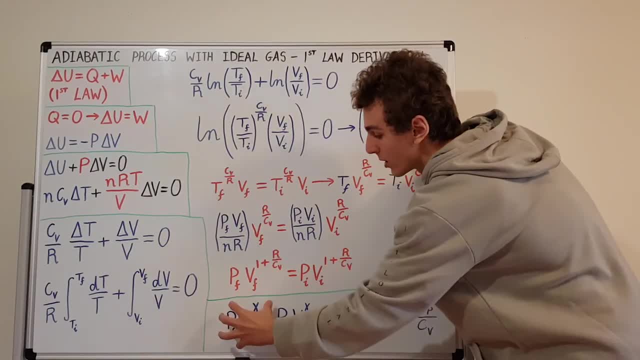 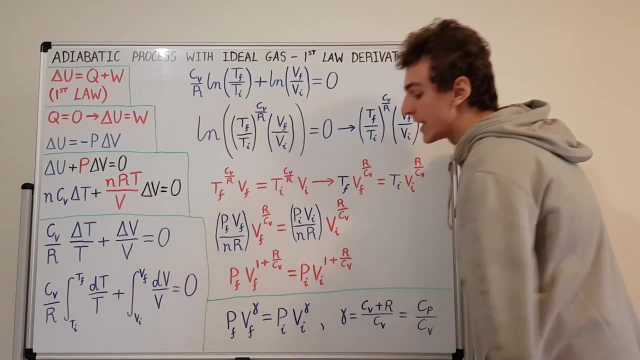 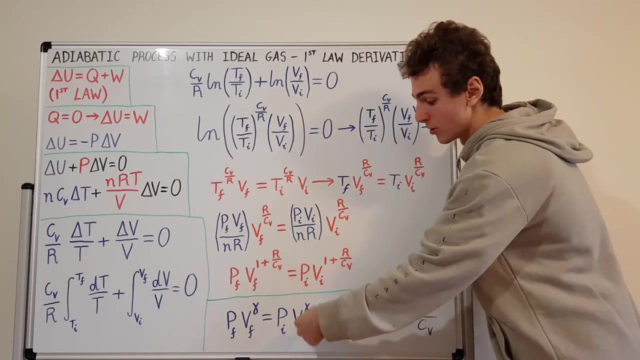 so anytime you see something like this, where you have some kind of product with a bunch of finals and a product and a bunch of initials in your subscripts, that is saying that this product is Constant at every point along the process. So if you take the beginning, which is the initial state, 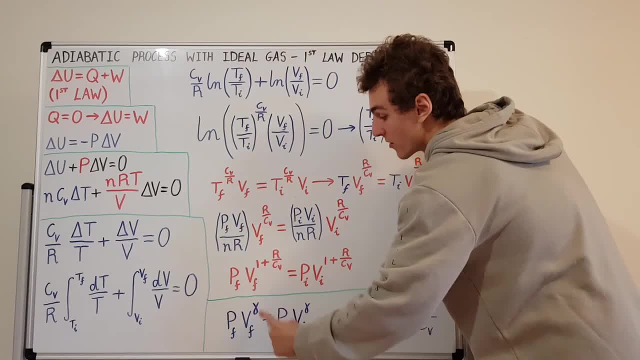 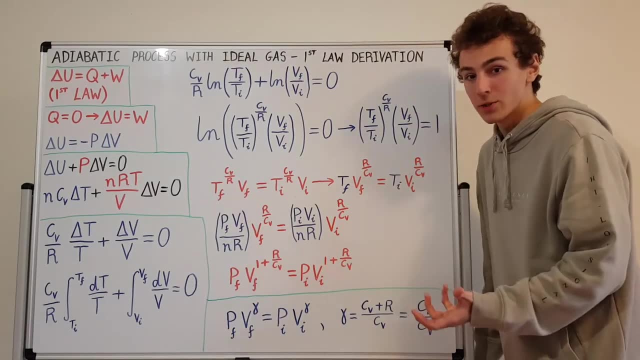 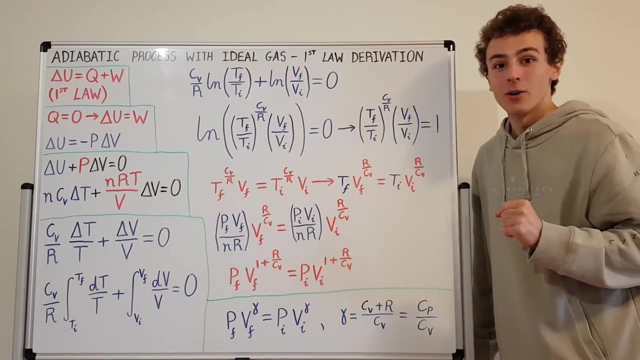 And then you continue at every intermediate state and you reach the final state that is going to be the same product. so for an ideal gas, where you're looking at an isothermal process, the isothermal process says that PV equals n or T and T is Constant. so P times V is constant, right? 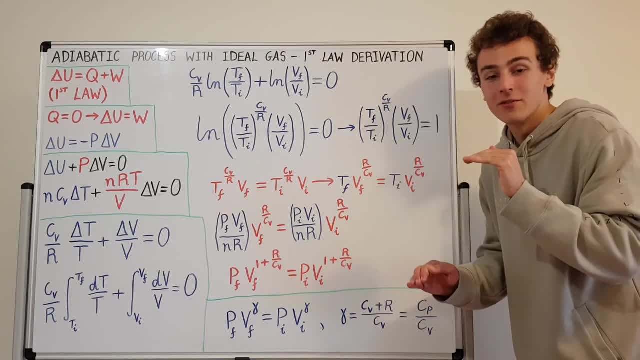 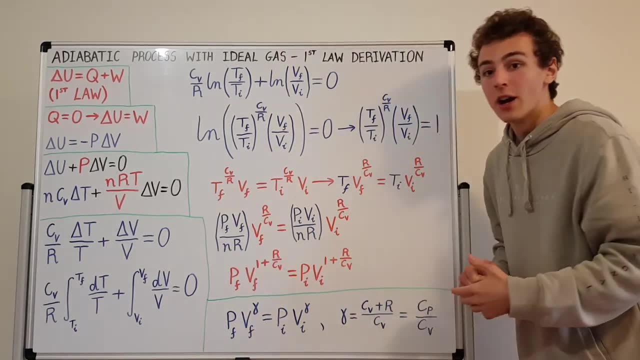 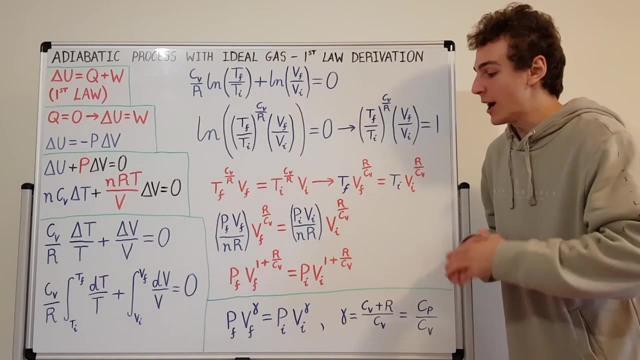 If P goes up, V must go down. if V goes up, P must go down. But in this case we don't have an isothermal process, We have temperature also changing right. temperature Can vary as well, so pressure can vary, volume can vary and temperature can vary. So how do we reconcile this? 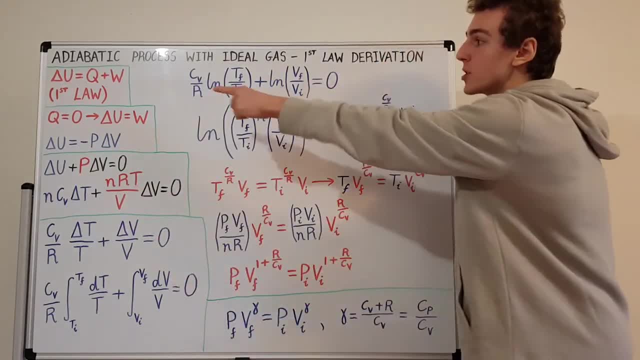 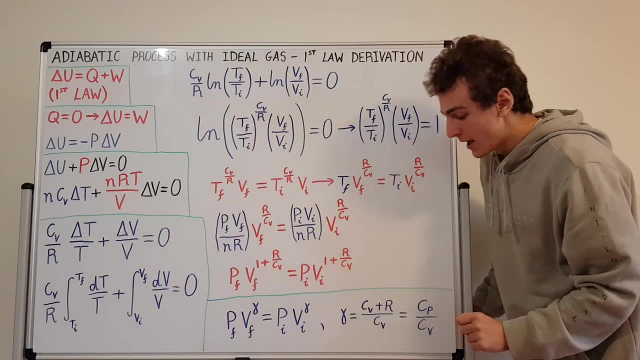 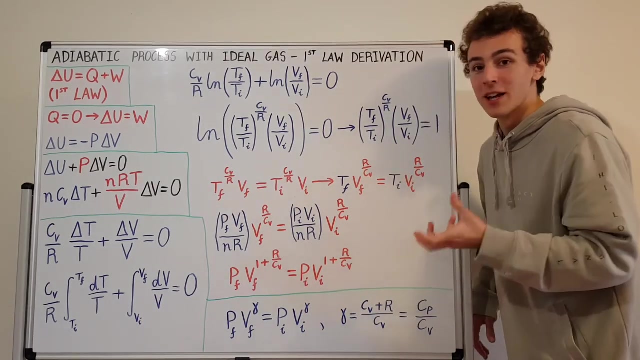 Well, we use this derivation using the first law of thermodynamics up there, and that gives us this lovely expression. Now, this gamma, this exponent, is actually linked to the degrees of freedom, right? So how many degrees of freedom, the part the particles have? so that's linked to whether they're monoatomic. 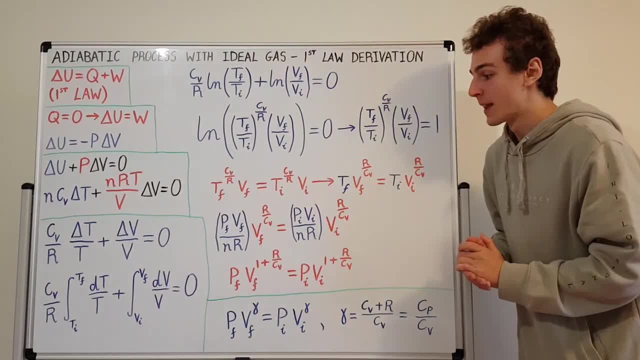 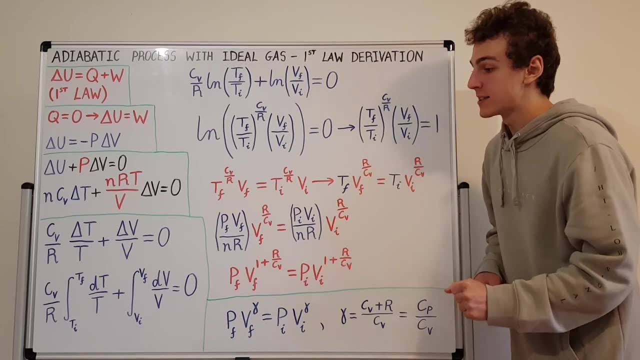 Diatomic, what kind of symmetries the molecules have. But keep in mind this is always for an ideal gas. So this derivation has been an adiabatic process with an ideal gas and we've used the first law of thermodynamics to get this. 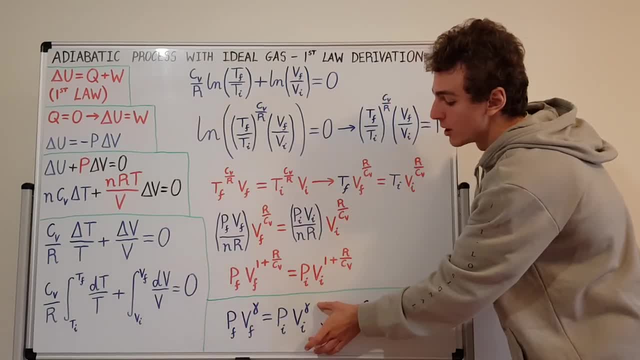 relationship, and this relationship is Absolutely essential to describing adiabatic processes on the PV diagram.